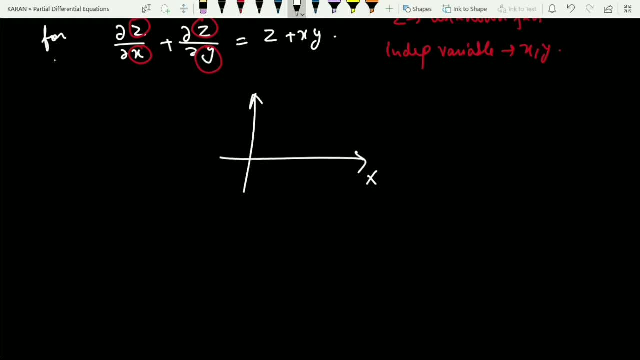 partial differential equation through a graph. For example, if this is my x-axis, this is my y-axis, fine, this is origin, and let a point here be a and here be point b. Now, for example, let us assume that here we have a string- fine, and a person is standing here and I have a touch test. 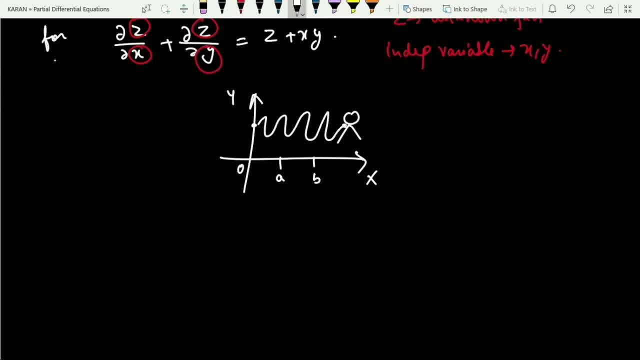 So I am going to put a string with his hand right now. once he start rolling out the string, once he start rolling this string, what will happen? the height with respect to of this string will change with respect to x-axis. So what I am trying to say is that height of the string with respect to x-axis. 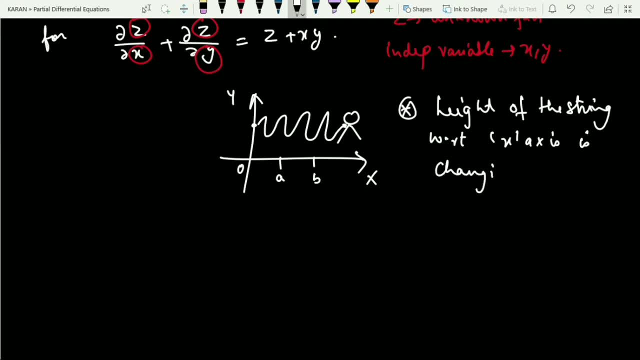 is changing. Yes, The height is changing, but with respect to what? with respect to x-axis is changing right, and that is with respect to time, also fine, and position also fine. For example, if you are at a, so the height is different. if you are at b, so the height is different, So the height of the string is. 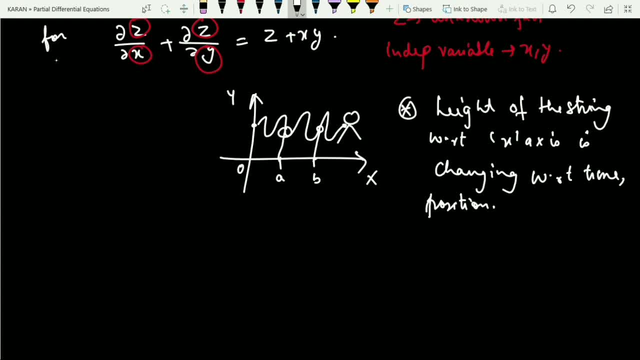 changing with respect to, you can say also with the time also, and we also with respect to position. So can I say, if I denote my height with u, so u will always come out to be a function of x and t. Fine, Yes, it is a having more than one independent. 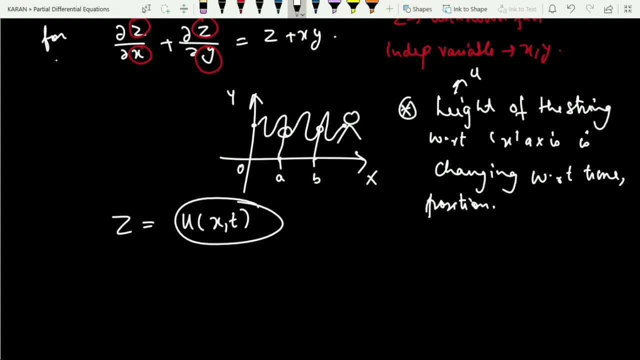 variable, so you can denote as z as a function of more than one variable, so it will again form partial differential equation. So here we have considered the example of a flexible string, fine, which was fixed with an end, fixed with the end. So, yes, you can see the example here Now. now let me 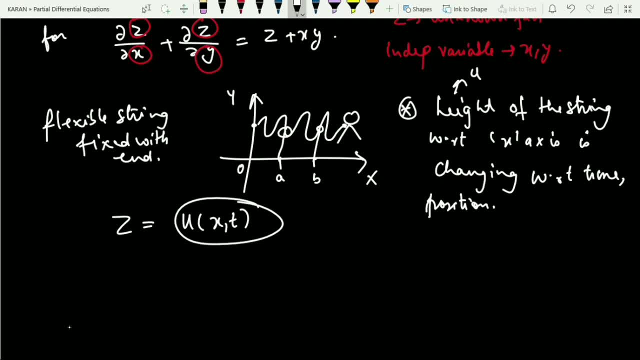 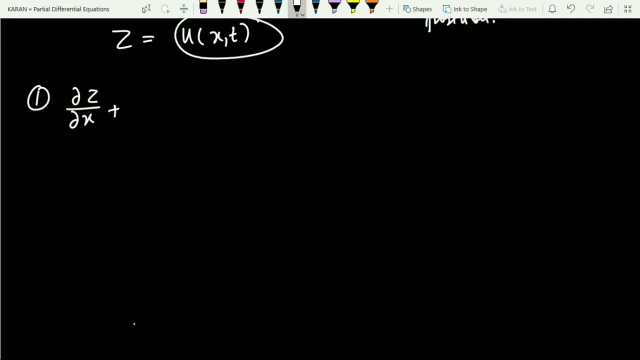 consider four to five more examples, and we will be considering those examples to study the further more results even So. the first example is del z by del x plus del z by del y, z plus x y. The second example is del z by del x, whole square. 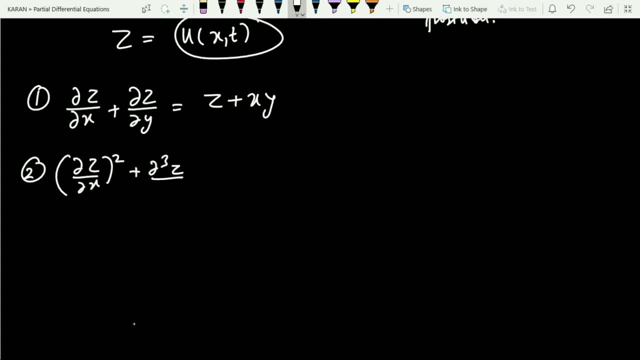 plus del cube, z by del y cube is equals to 2, x del z by del x. The third one is z into del z by del x plus del z by del y is equals to x. The fourth one is del u by del x plus del u by del y plus del u by del z. 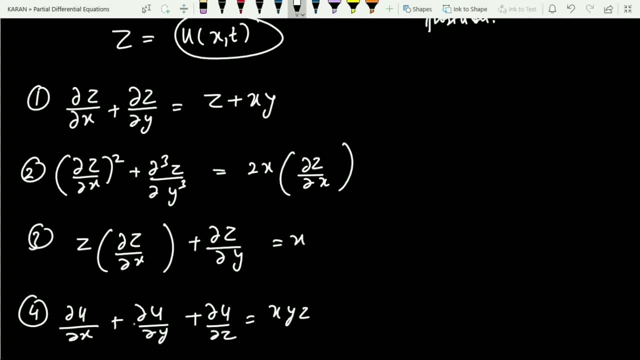 equals to x, y and z. And let me write: the fourth one is here. The fourth example is del square z, So it's fifth one. So the fifth example del square z by del x square is equals to 1 plus del z by del y. 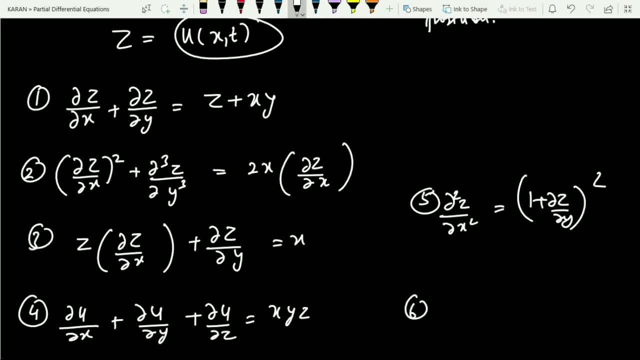 full whole square. And the last one is y times del z by del x whole square plus del z by del y whole square is equals to z into del z by del y. So here I have shown you the six examples, which are the examples of a partial differential equation. Now why I have written these examples, it will be more. 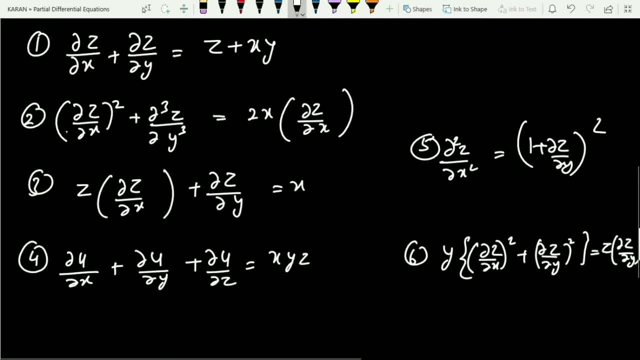 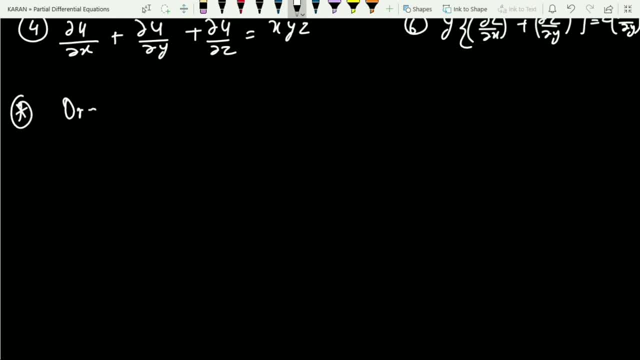 clear once we discuss the definition of your order and degree, and then I'll be explaining that. what is the order and degree of a partial differential equation? So let's start with the order and degree of these six examples. So now, next definition that comes out to be is order of a. 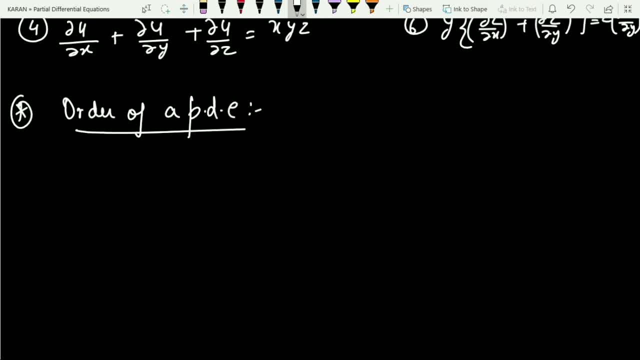 partial differential equation. So when we talk about the order of a partial differential equation, it is nothing but the order of a highest partial derivative. So it is the order of a highest partial derivative occurring in the differential equation. So occurring in my partial differential equation. Fine. So now let us see. 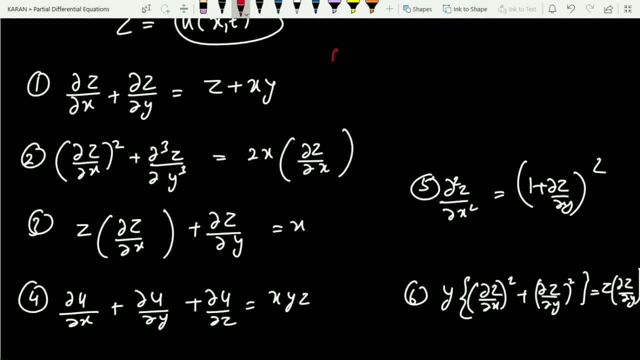 For example, the first example. coming on to the first example, now we will be writing the order. So my definition of order states that order of a highest partial order derivative. So the highest partial derivative is one only in this case. Fine. What about the second example In the second? 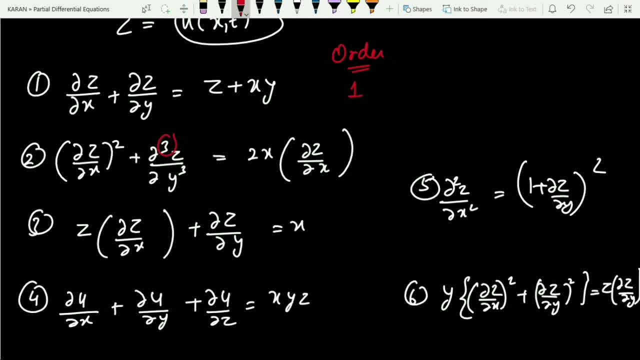 example, you can easily see that the highest order is 3.. Fine, So the order comes out to be 3 in this case. Come to the third example. Similarly, the highest order is just 1 out of any partial derivative, So order is 1 in this case. Similarly, in the fourth example also, it is 1. Fine, Come on moving on. 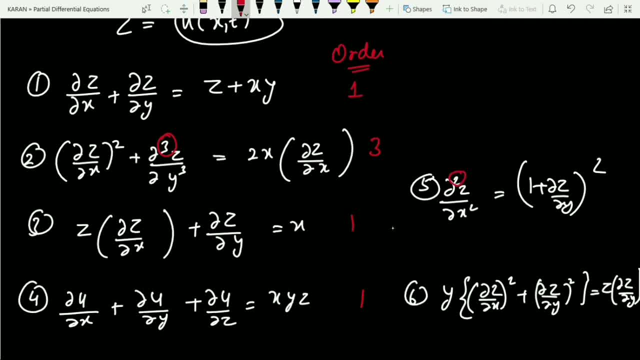 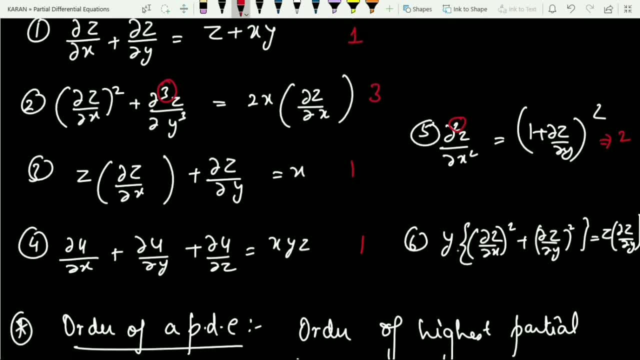 the fifth example You can see here it is dell square, Fine, So the order comes to be 2 in this case. and the last example is nothing but by the highest order. partial derivative here also is of order 1, fine, so the order will come out to be 1. do not confuse that. this is uh, del x by del. 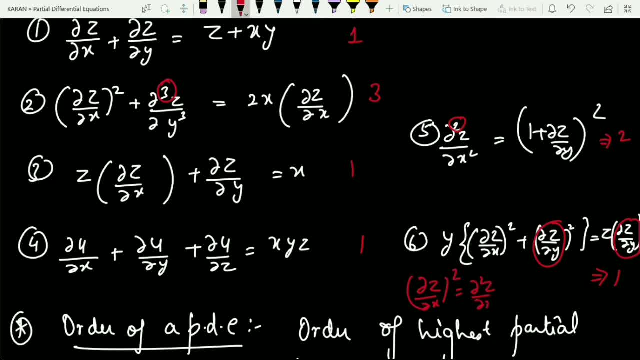 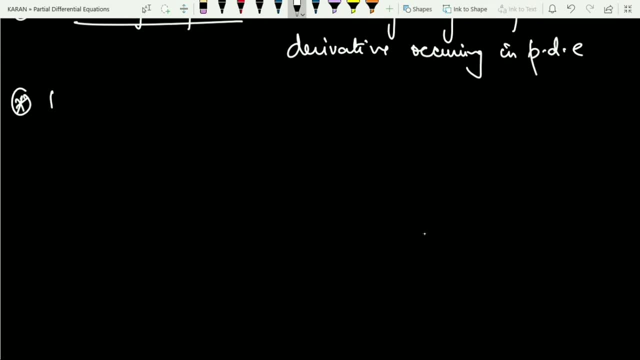 x whole square is equals to del square z by del x squared. so these are not equal. so do not tell me that the order of this equation is 2. fine, so they are not equal now. now let us discuss the definition of a degree. what is a degree of a partial differential equation? so the degree of a. 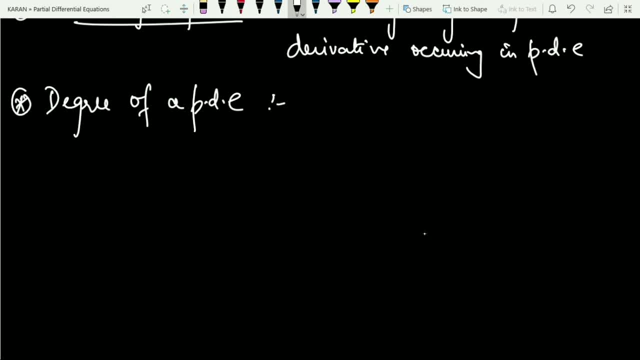 partial differential equation. so when we talk about the degree, it is nothing but the. it is the degree of highest order derivative which occurs in it, which occurs in it r after the equation has been rationalized. after the equation has been rationalized. so when i say that the equation has been rationalized, what does it mean? 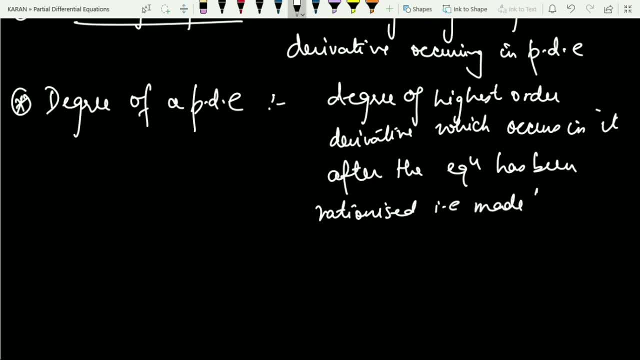 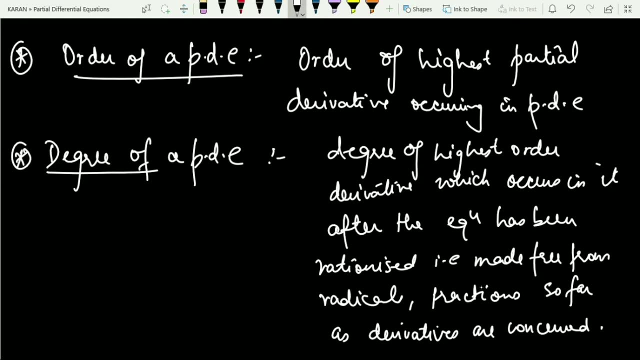 it means that it is made free from radicals. radicals as well as you know. fractions, so fractions so far as the derivatives are concerned. so the degree of a partial differential equation is nothing, but the degree of a partial differential equation is the degree of the highest order derivative which occur in the equation. 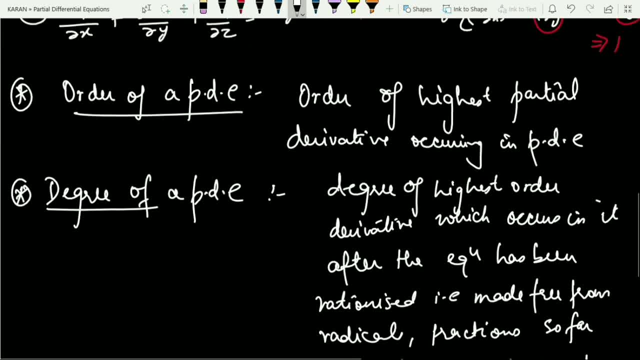 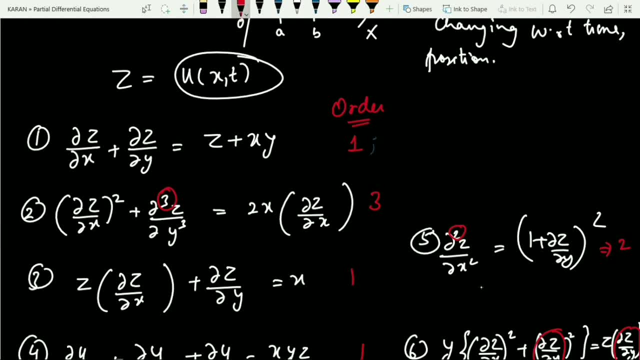 once the equation has been rationalized. so let us see what is the degree of the various partial differential equations here. fine, so you know that the highest order derivative was 1 here, and what is the power? that is 1. so the degree in case of first equation will be: 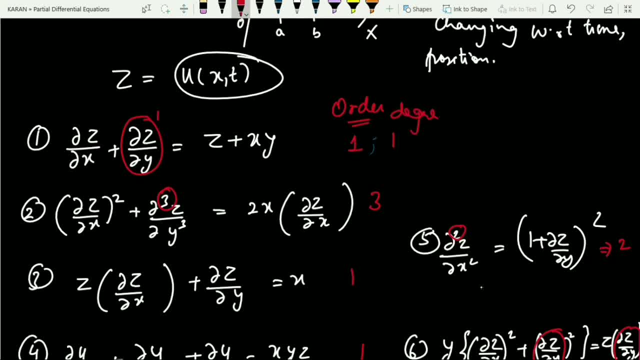 1. fine, so here i am writing with degree now. now moving on to the second equation. so the highest order derivative was 3, and what is the power of that? again, that is 1. so the degree in this case is also 1. what about third example? so again, the degree will be 1. and in the fourth, 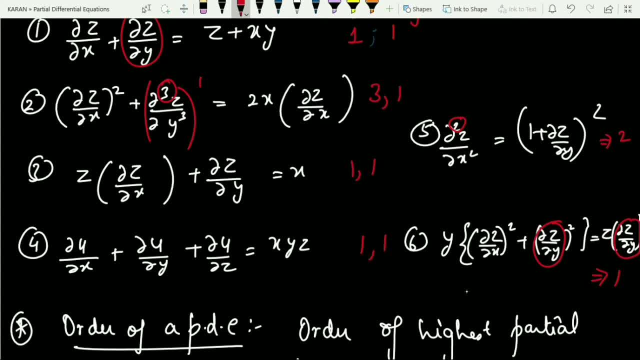 example also the degree will be 1. but in fifth example, just observe. so once you open this, so this will be del square x by del x, square, fine. this is 1 plus del z by del y, whole square, fine, plus twice del z by del y. so clearly the degree also in this case is 1. and in the last case what? 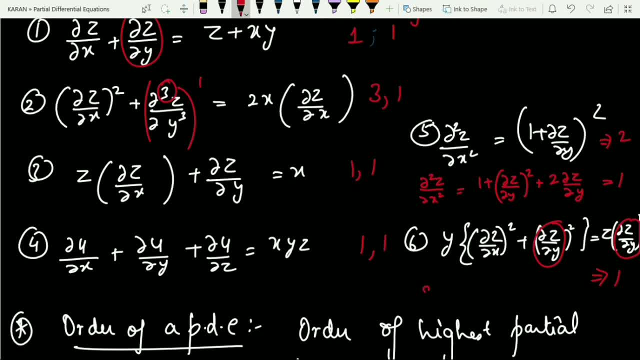 is the degree. so you can easily see that the degree here will be 2. now why it will be 2? because you can easily see that the power of this del z by del y is 2, so that is the degree of the partial differential equations. so i hope both these definitions are clear till now. now let us move. 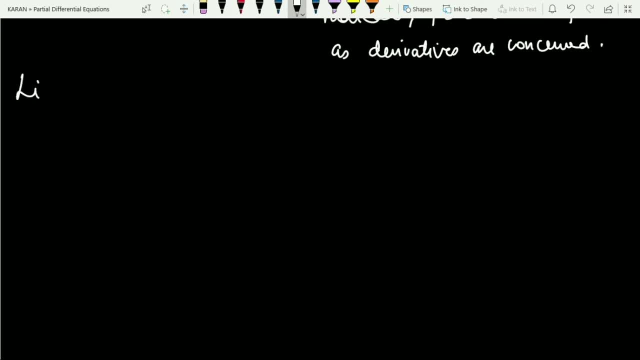 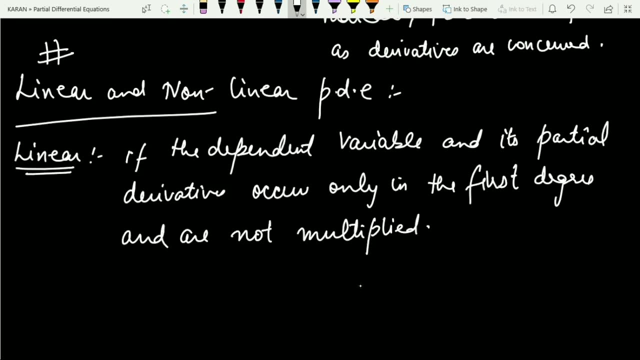 to the definition of linear and non-linear. so linear and linear and non-linear, non-linear, partial differential equations. so it is defined. any equation, any pd is said to be linear if the dependent variable- i hope you know what is the dependent and independent- if i say del z by del x, so this is a dependent variable, fine, and this is a independent variable, fine. 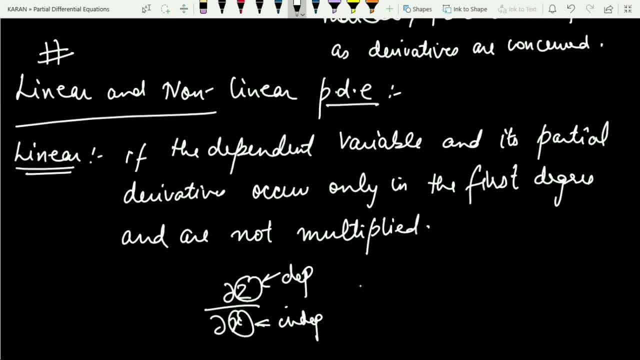 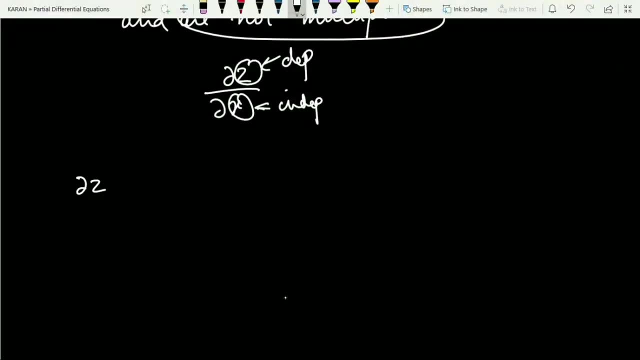 so if the dependent variable and its partial derivatives occur only in the first degree, fine, and they are not multiplied with each other, fine. you can easily observe that. my first example. so what is my first example? i will write it again. so the first example was: del z by del x plus del z by del y is equals to z plus x y. so you can clearly. 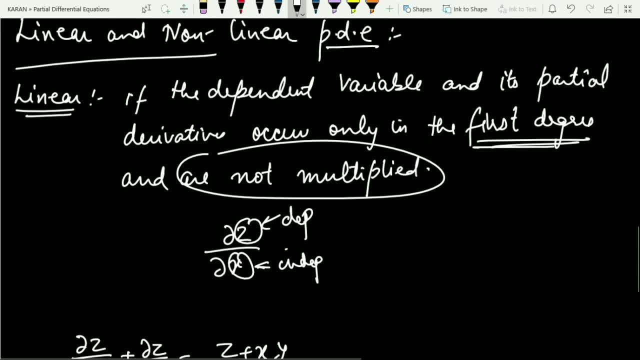 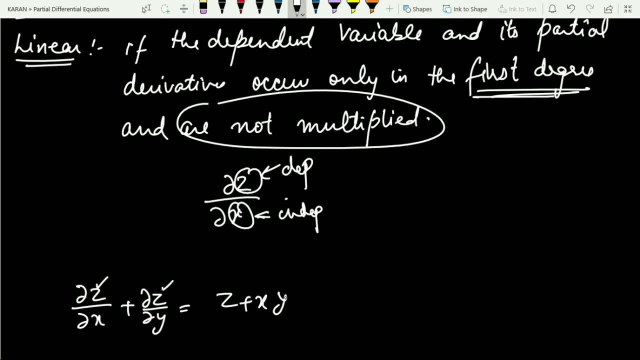 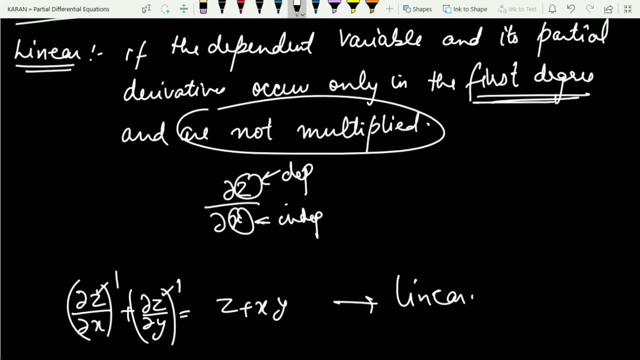 observe that the dependent variable. so this is a linear equation. why? because because the dependent variable, that is z- fine, and its partial derivatives occur only in the degree 1- fine, and they are not multiplied with each other. so, yes, this is a linear differential equation. now, going back, let us see which all equations are linear or not. so my first equation is linear. 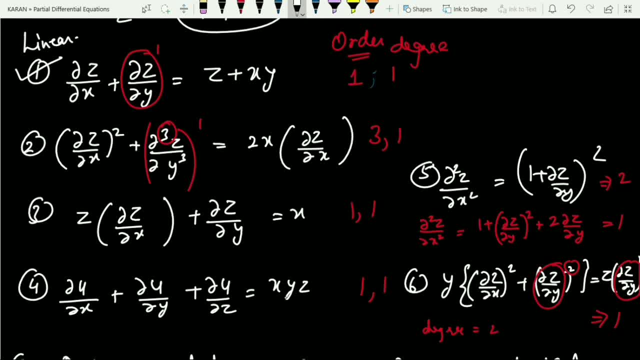 what about the equation number two? the equation number two is a non-linear. why it is a non-linear? because you can see that my dependent variable and its partial derivatives are multiplied with each other. so this is a non-linear. fine, so the equation which is not linear, that is called as a. 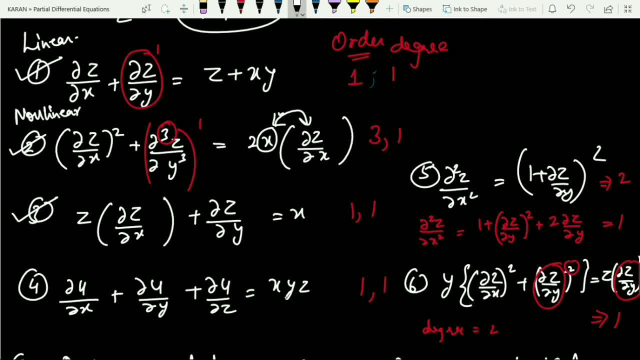 non-linear differential equation. similarly, third will also be non-linear, because z is multiplied with del z by del x. fine, and what about the non-linear differential equation? so this is a non-linear differential equation. what about fourth? fourth is a linear differential equation. fine, so this is a linear. and this was. 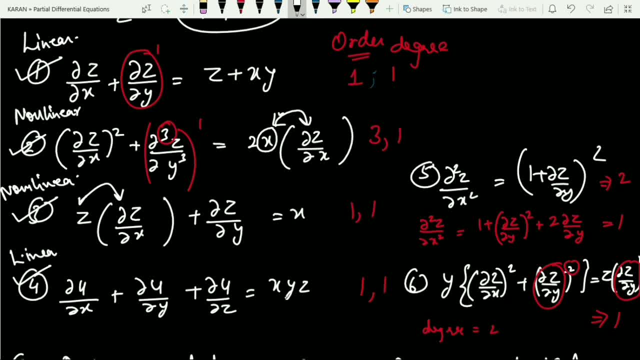 non-linear. again, the fifth one is a non-linear because the degree is two. so this is a non-linear. fine, and what about the sixth one? and similarly, the sixth one is also the non-linear partial differential equation. so i hope again, linear and non-linear differential equations is also clear. 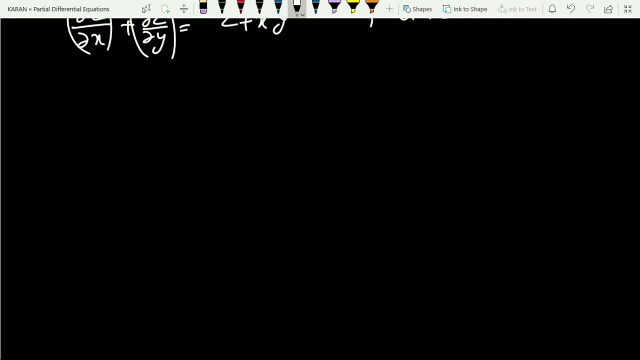 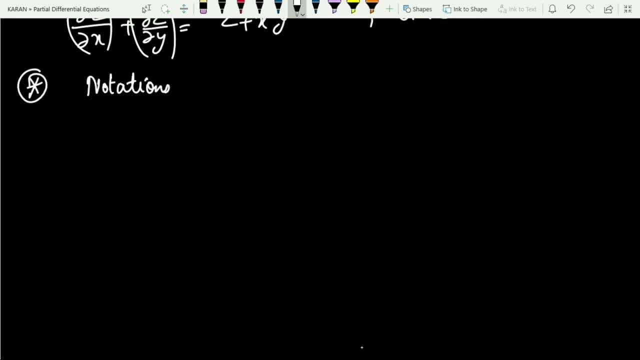 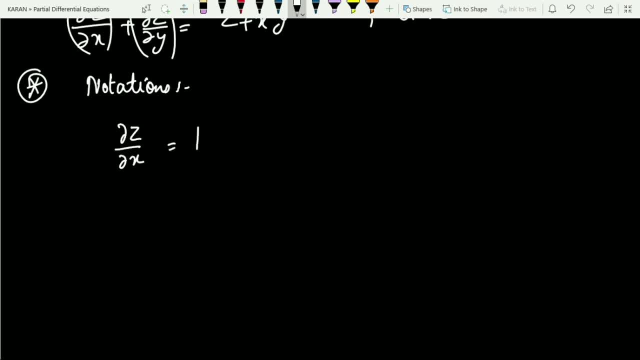 will be using are so: whenever i have to denote del z by del x, i will be writing it as del z by del x, i will be writing it as del z by del x, i will be writing it as p. if i have to denote del z by del y, 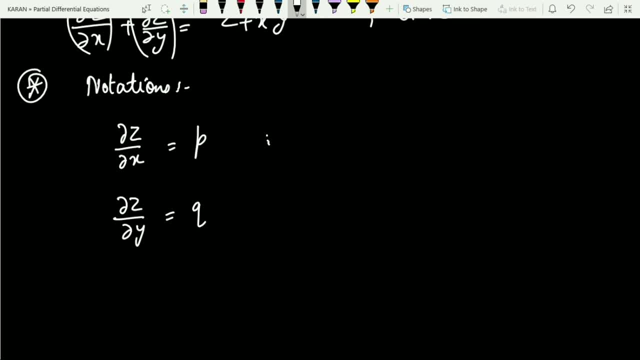 p. if i have to denote del z by del y p. if i have to denote del z by del y, i will be writing it as q fine. and if i, i will be writing it as q fine. and if i, i will be writing it as q fine. and if i have to denote del square z by del x. 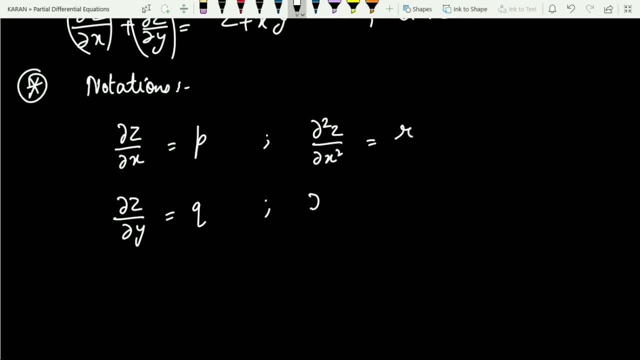 have to denote del square z by del x, have to denote del square z by del x square, i will be denoting it with r square. i will be denoting it with r square, i will be denoting it with r. and if i have to denote del square z by 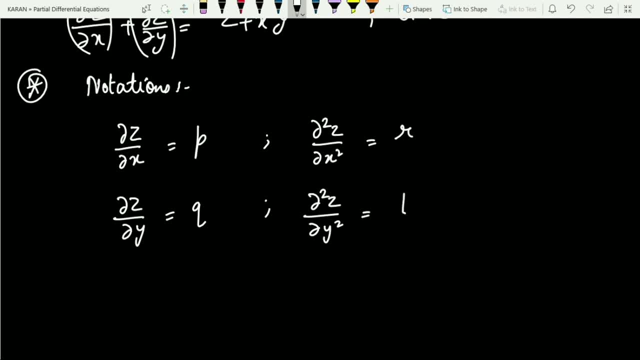 and if i have to denote del square z by, and if i have to denote del square z by del y square, del y square, del y square, i will be denoting it with t and last. if i will be denoting it with t and last if 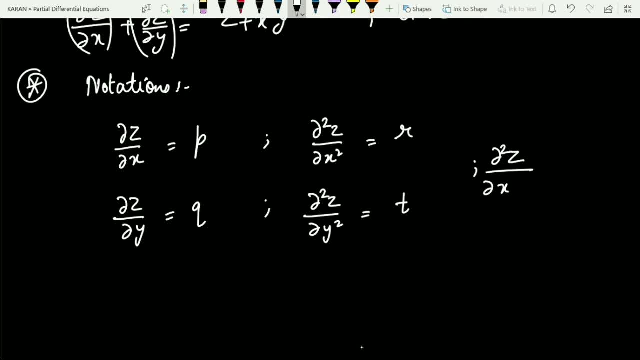 i will be denoting it with t. and last, if i have to denote del square z upon, i have to denote del square z upon. i have to denote del square z upon del x del y, so i will be denoting it. del x del y, so i will be denoting it. 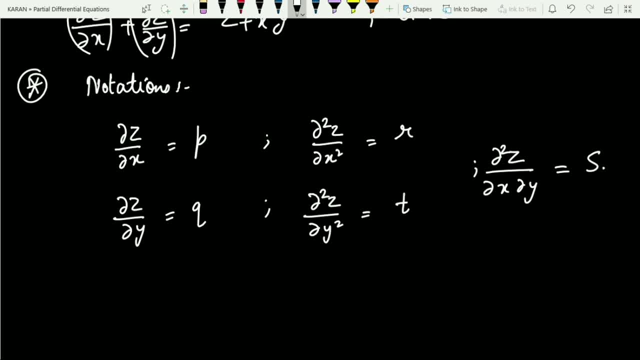 del x, del y, so i will be denoting it with s. so these are basically the five with s. so these are basically the five with s. so these are basically the five notations which i will be considering, notations which i will be considering, notations which i will be considering throughout my video lectures, and you. 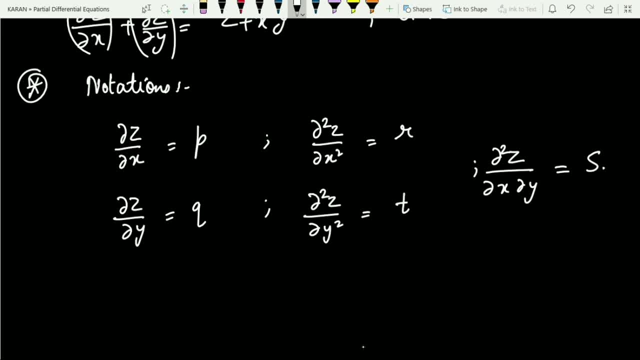 throughout my video lectures and you throughout my video lectures and you should be familiar with these, should be familiar with these, should be familiar with these notations. fine, now in case, if we have notations. fine, now in case, if we have notations. fine, now in case, if we have n independent variables, and i take the 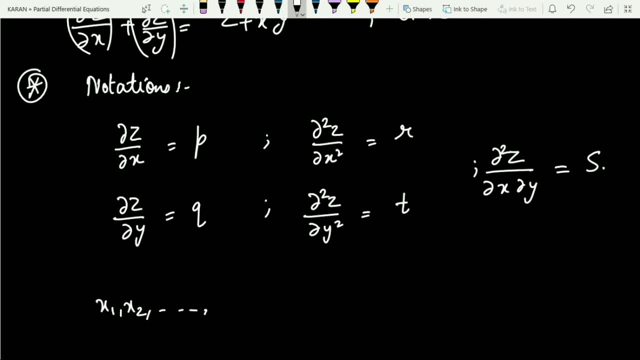 n independent variables and i take the n independent variables and i take the independent variables to be x1, independent variables to be x1, independent variables to be x1, x2 and so on. to xn- fine and z is x2, and so on. to xn- fine and z is. 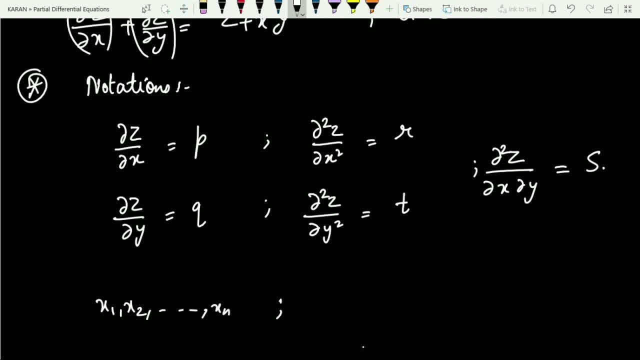 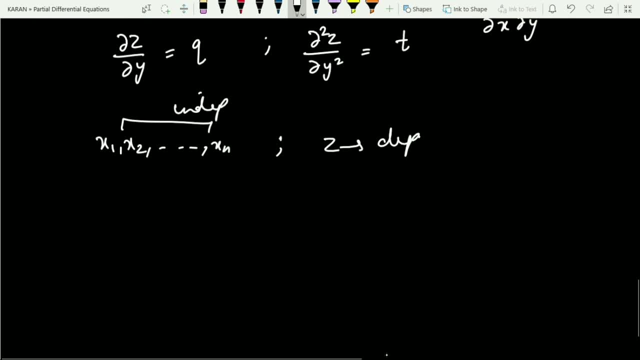 x2 and so on to xn. fine, and z is regarded as a dependent variable fine regarded as a dependent variable fine regarded as a dependent variable fine, and these are my independent variables, and these are my independent variables- fine and so on to xn. so this is again. 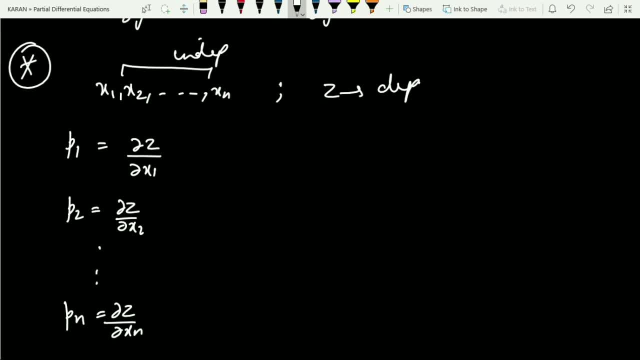 fine, and so on to xn. so this is again fine, and so on to xn. so this is again one of the notation which i will be, one of the notation which i will be, one of the notation which i will be considering in the considering, in the considering, in the upcoming lectures. and the last thing: 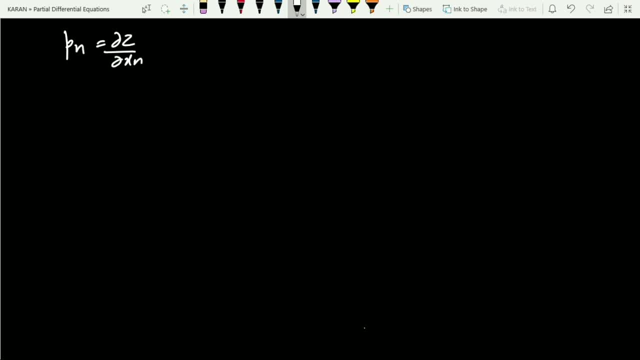 upcoming lectures and the last thing: upcoming lectures, and the last thing which i will sometimes i will be using, which i will sometimes i will be using, which i will sometimes i will be using in the suffixes, that is, if i have to in the suffixes, that is, if i have to. 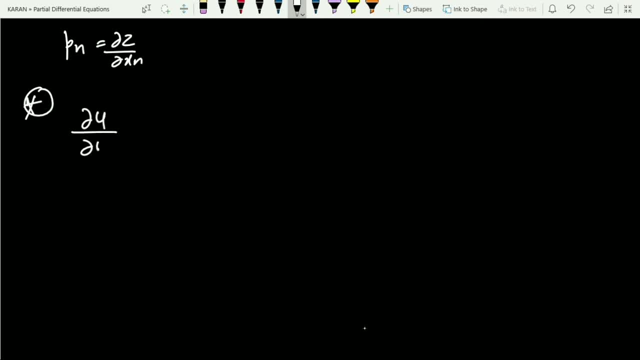 in the suffixes, that is, if i have to denote denote, denote del u by del x, fine. so del u by del x, so del u by del x, so del u by del x. so it could be written as u x u sub x. fine, it could be written as u x u sub x, fine. 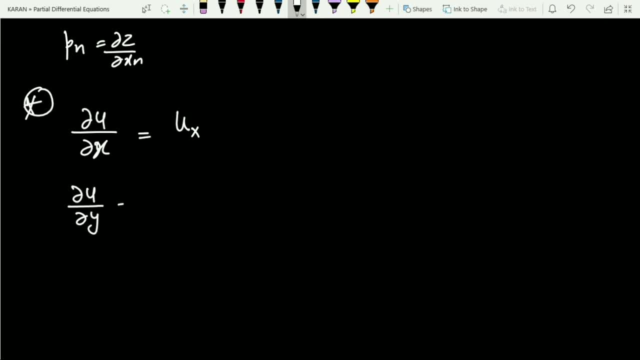 it could be written as u x, u sub x. fine, this is a suffix. similarly del u by del. this is a suffix. similarly del u by del. this is a suffix. similarly del u by del y, y, y. sometime it will be denoted as u, y and. 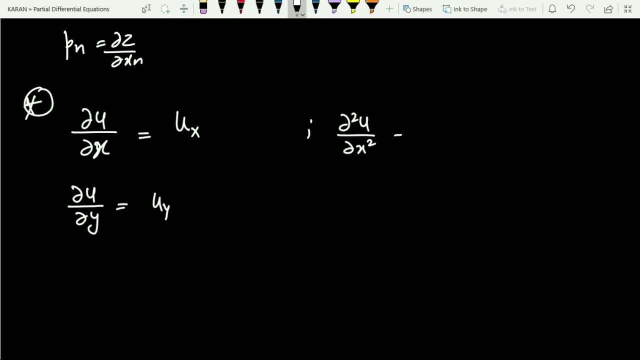 sometime it will be denoted as u y and sometime it will be denoted as u y, and if i have to say del square u by del x, if i have to say del square u by del x, if i have to say del square u by del x square, so it could be denoted as: 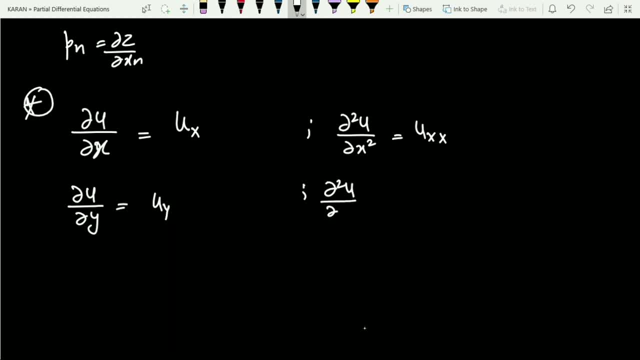 square, so it could be denoted as square. so it could be denoted as u x x. fine. similarly del square u. u x x, fine. similarly del square u. u x x, fine. similarly del square u. by del y square, so it would be denoted by del y square. so it would be denoted. 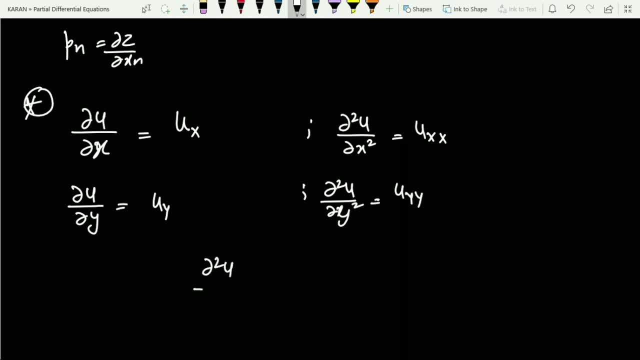 by u y y, and the last one is del square u by u y y, and the last one is del square u by u y y, and the last one is del square u del x del y, so this will be denoted as u del x del y, so this will be denoted as u. 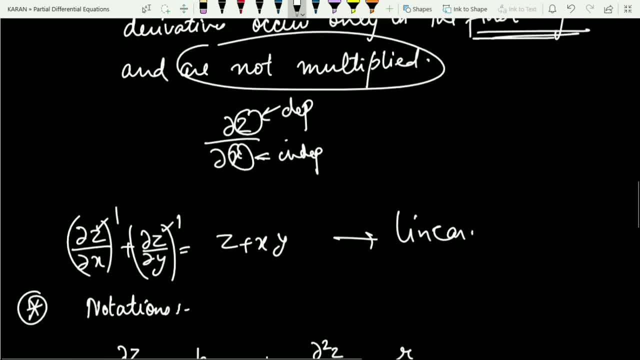 del x, del y. so this will be denoted as u x y. so these are the notations which i x y. so these are the notations which i x y. so these are the notations which i will be considering. the will be considering the will be considering the upcoming video lectures, so i hope the 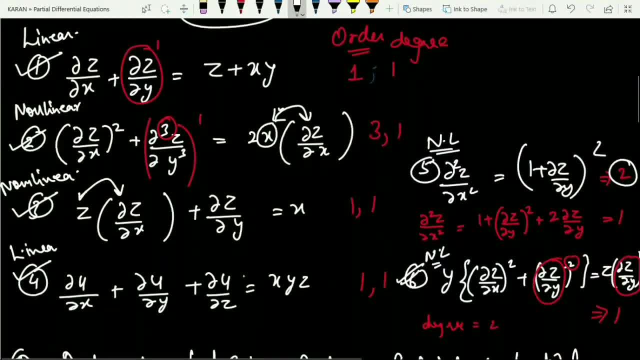 upcoming video lectures, so i hope, the upcoming video lectures, so i hope. the definitions, definitions, definitions of the partial differential equation. what of the partial differential equation? what of the partial differential equation? what is the order? is the order? is the order? what is the degree? what is a linear and a? 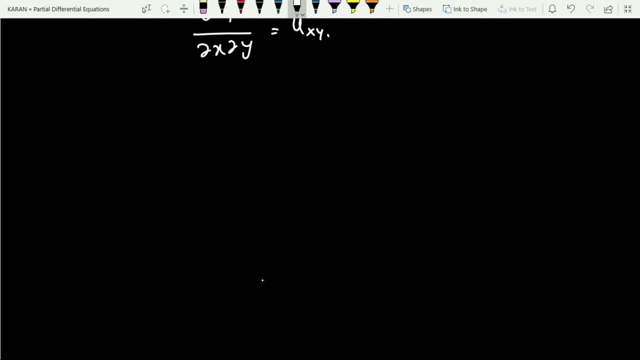 what is the degree? what is a linear and a? what is the degree? what is a linear and a non-linear differential equation is non-linear. differential equation is non-linear differential equation is clear to you in the upcoming video. clear to you in the upcoming video. clear to you in the upcoming video lectures. we will be classifying the. 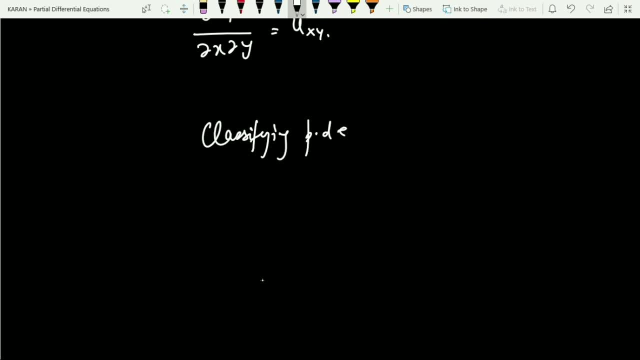 lectures. we will be classifying the lectures. we will be classifying the partial differential equations first of partial differential equations, first of partial differential equations, first of all, and then we will learn how to all, and then we will learn how to all, and then we will learn how to formulate or how to derive partial 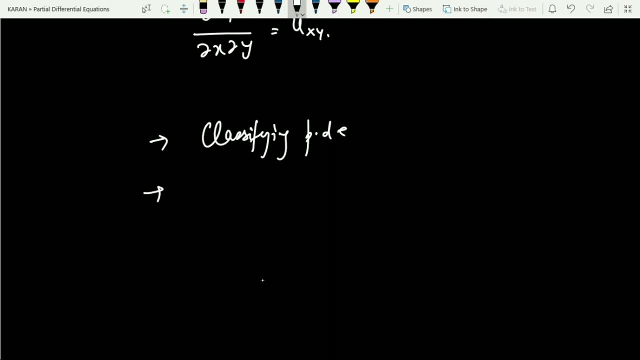 formulate or how to derive partial formulate or how to derive partial differential equations by elimination, differential equations by elimination, differential equations by elimination, eliminating the arbitrary constants and eliminating the arbitrary constants and eliminating the arbitrary constants. and in the upcoming lectures we will be. in the upcoming lectures we will be. 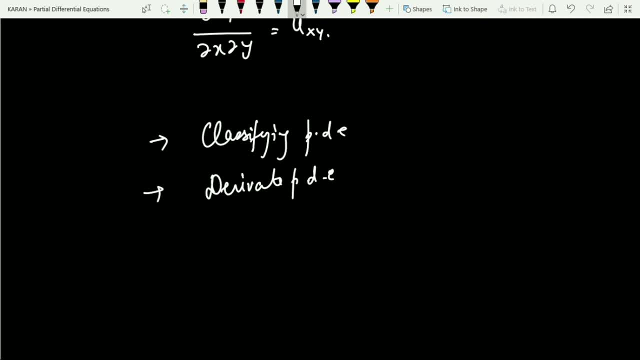 in the upcoming lectures we will be considering many examples so that the considering many examples, so that the considering many examples, so that the things are clear to you in more familiar, things are clear to you in more familiar, things are clear to you in more familiar way. so I hope you have understood this. 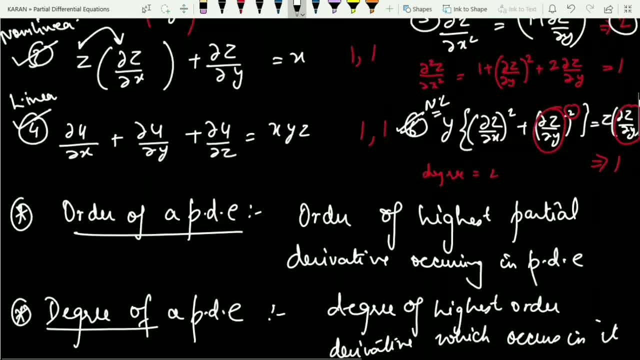 way. so I hope you have understood this way. so I hope you have understood this video lecture. you can go home and video lecture. you can go home and video lecture. you can go home and practice more and more questions which practice, more and more questions, which practice more and more questions which are based on order, degree and linearity. 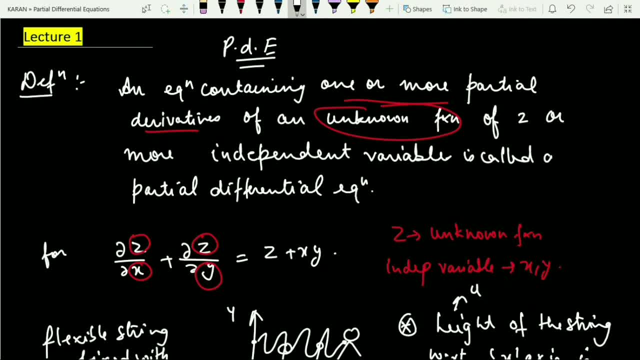 are based on order, degree and linearity are based on order, degree and linearity and if you face any doubts, you can, and if you face any doubts, you can, and if you face any doubts, you can mention your doubts in the comment box. mention your doubts in the comment box.